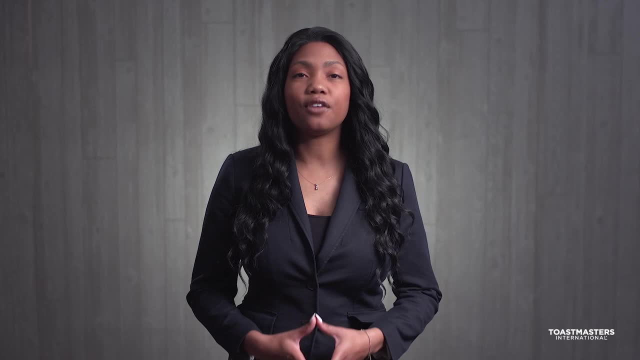 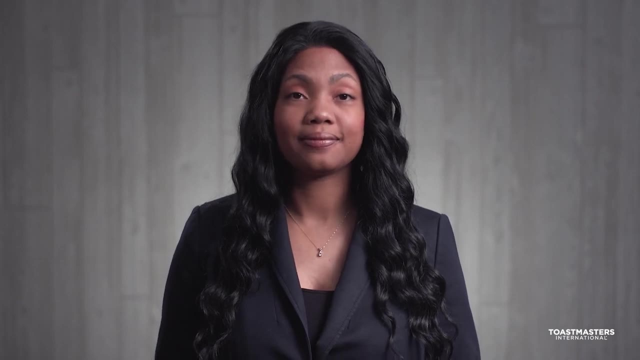 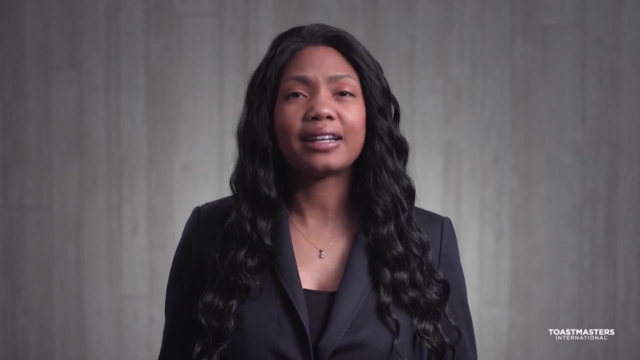 And you won't have to struggle to keep your messages straight if you know the message well. Once you've mastered your topic, you need to master your presentation. Make sure you rehearse the entire speech so you will be more comfortable presenting it, And practice any difficult parts repeatedly until they flow smoothly. 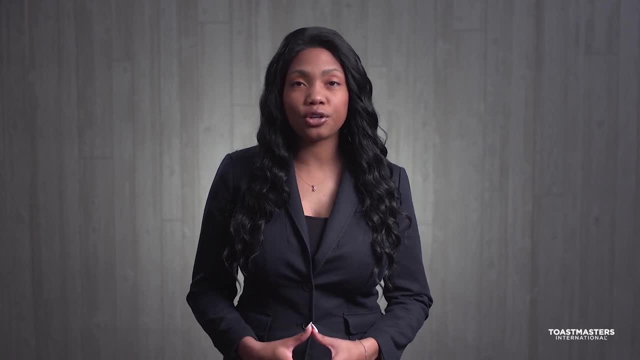 Whether or not you memorize each word. it's up to you to decide whether or not you're going to be able to follow the order of your messages. That's why new Toastmasters members begin with the icebreaker speech. It's a chance to talk about the subject you know best—yourself. 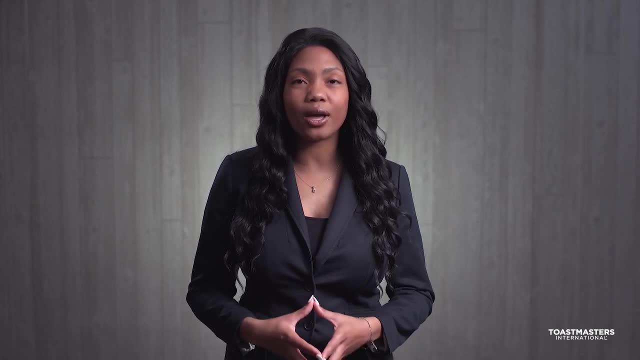 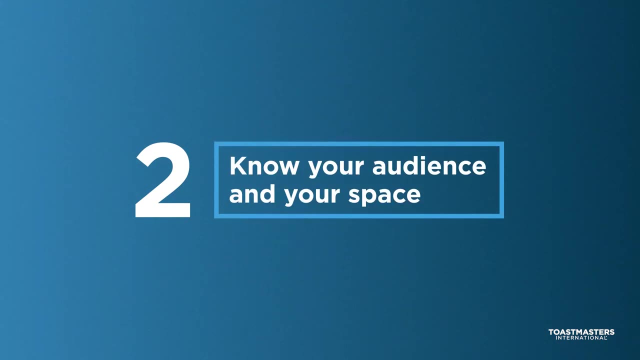 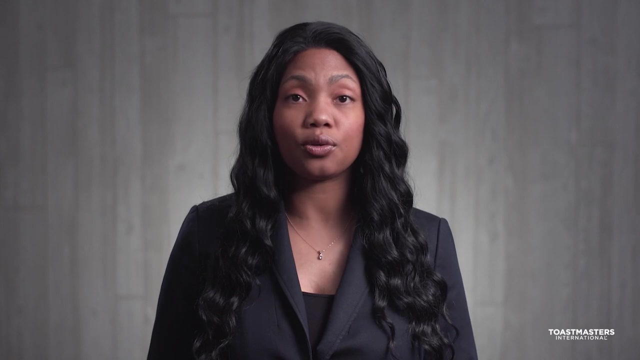 Then all you have to focus on is practicing how well you tell your story. 2. Know Your Audience and Your Space. Understand the importance of your audience. Understand the importance of knowing who will be listening to you and where you will be when you give your presentation. 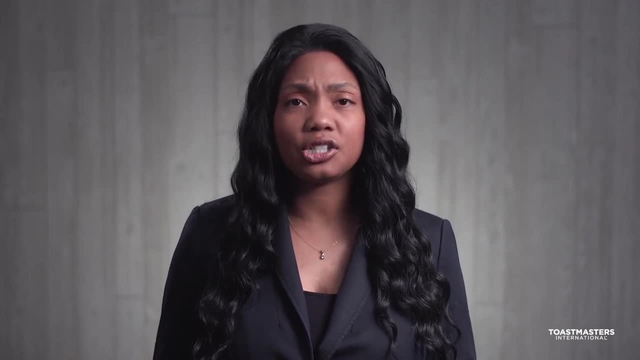 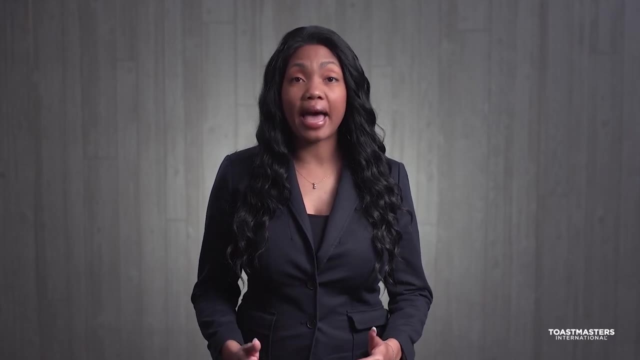 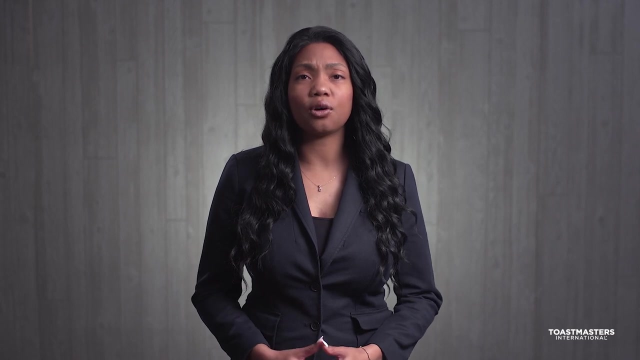 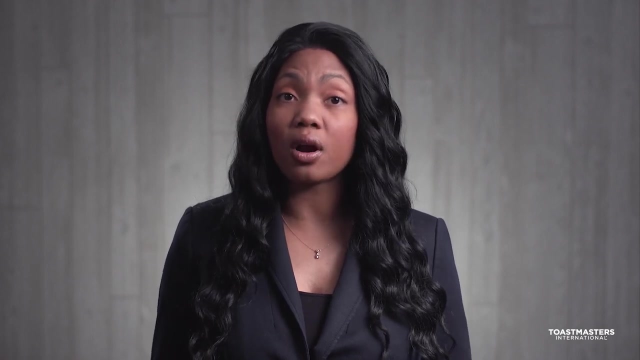 Both the audience and location can create limitations that are important to understand. For example, a researcher might speak about the math behind their work. If they're addressing a group of college professors, they could use highly technical language to discuss a sophisticated project. But would they want to do that if they were describing their work to a group of elementary? 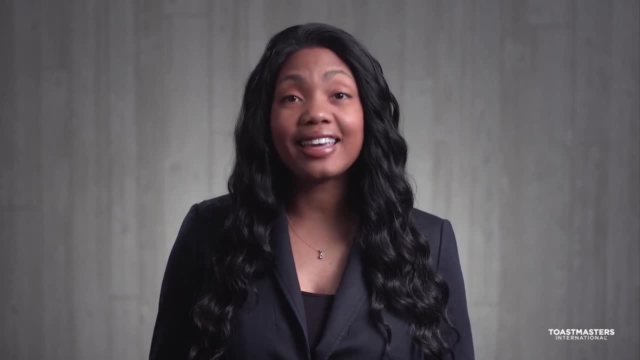 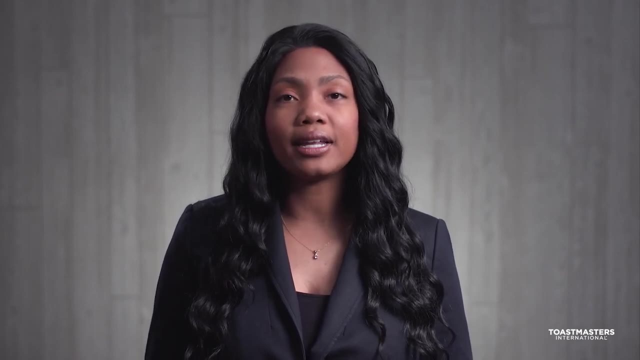 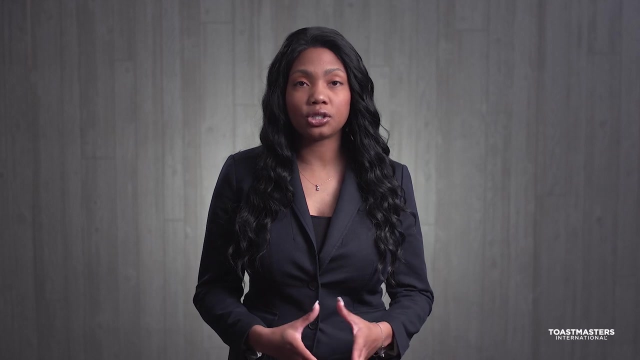 students, Of course not For young kids. it would be better to talk about how we learn through the research process. Knowing your audience means understanding and respecting their particular characteristics Before you prepare your speech. their geography, politics, culture, age and other traits will 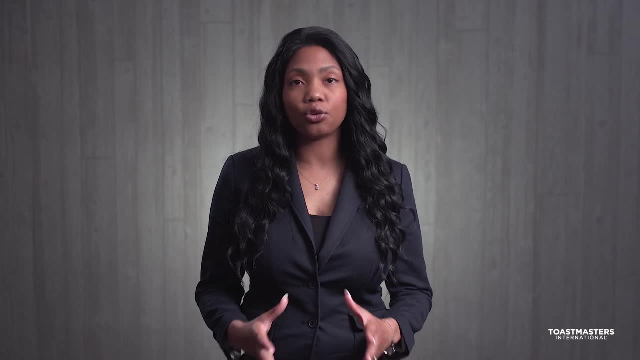 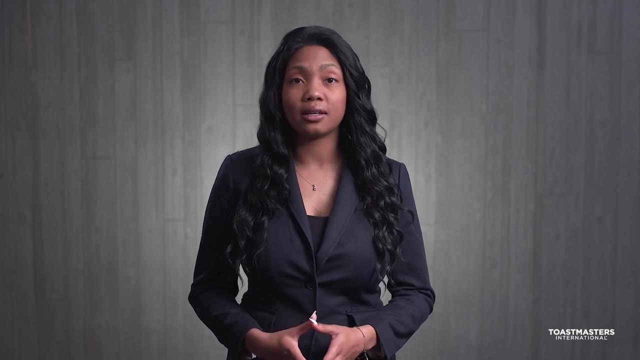 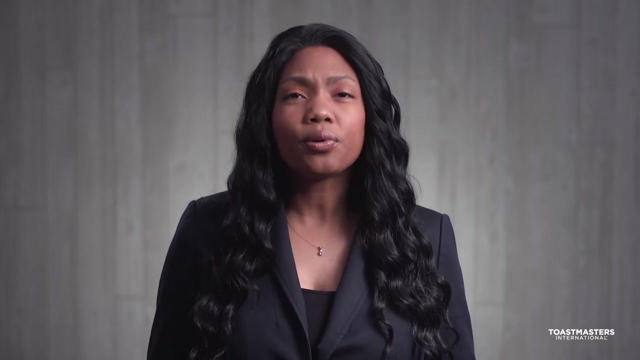 define them as a group and will guide you in tailoring your presentation to fit their needs. Preparation reaches beyond understanding your audience. You need to also consider how they will experience your speech. For example, when you present to an in-person audience, be sure to check out your location. 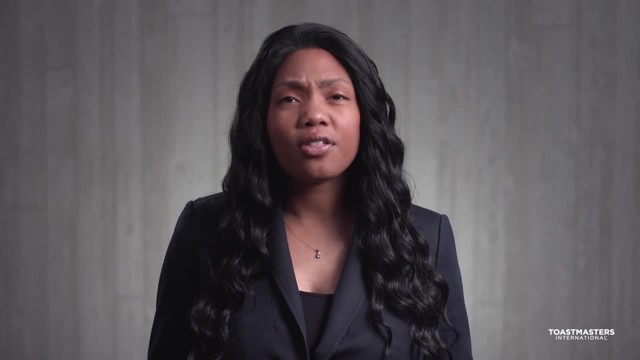 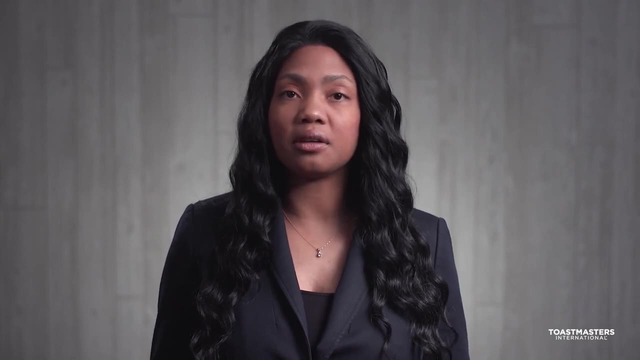 before the event begins: Will there be enough space on stage for everything you need? 3. If you're planning to use any media that requires a monitor or a screen, is the venue aware? Do they have everything you require? If your presentation will be online or hybrid, have you learned everything you need to know? 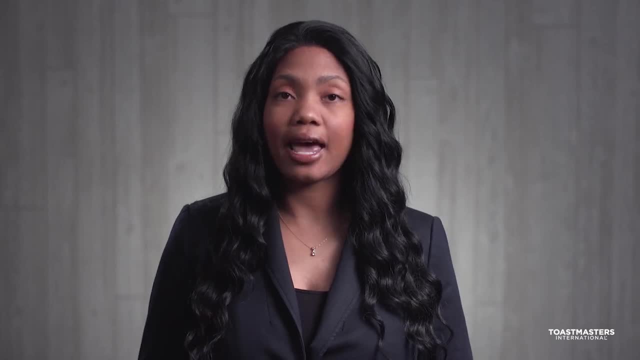 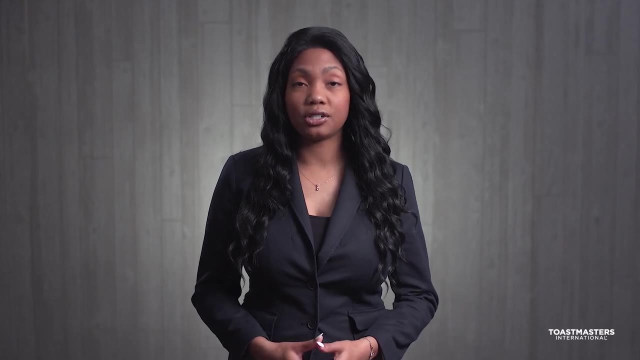 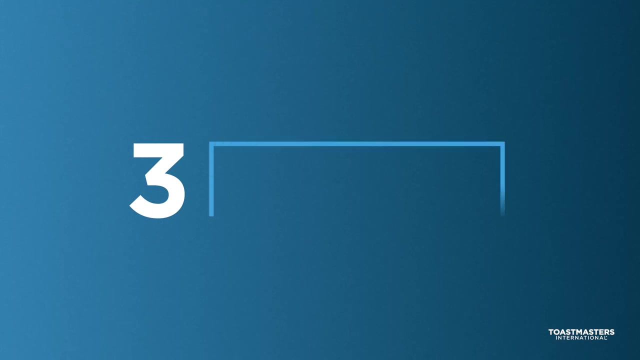 about the app you will use. Can you access chat? Will it be turned off or will someone else facilitate that feature for you? All these questions are important to answer before you start your presentation. 4. Keep going. There's no need to apologize if you make a. 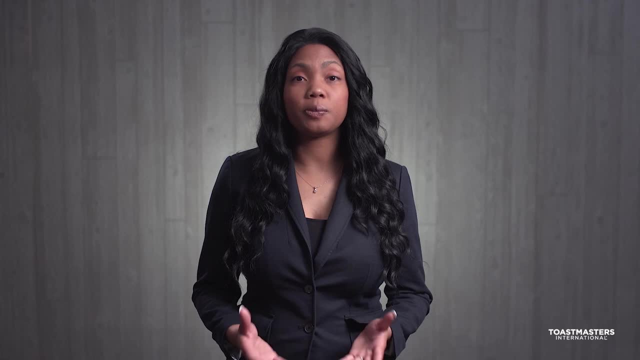 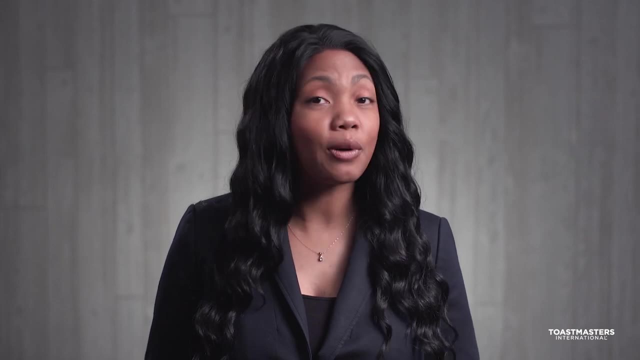 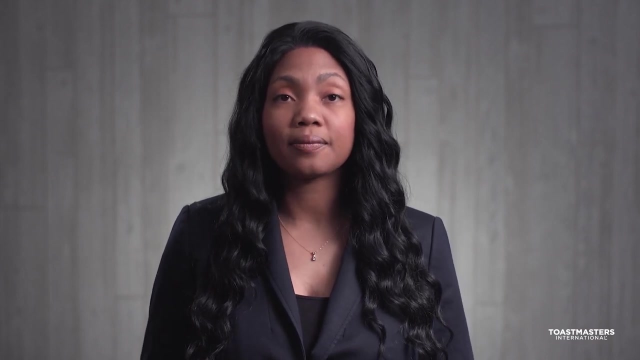 minor mistake, such as skipping a portion of your speech or forgetting a few words. If something like this happens, don't worry. Your audience most likely doesn't know the difference. Just move on and you'll find your way back on track with your next point. 5. If you apologize, you're not going to make a difference. 6. If you apologize, you're not going to make a difference. 7. If you apologize, you're not going to make a difference. You call attention to the mistake, which takes away the important point you want to. 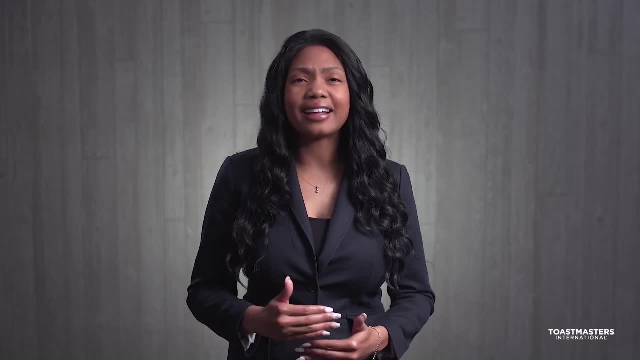 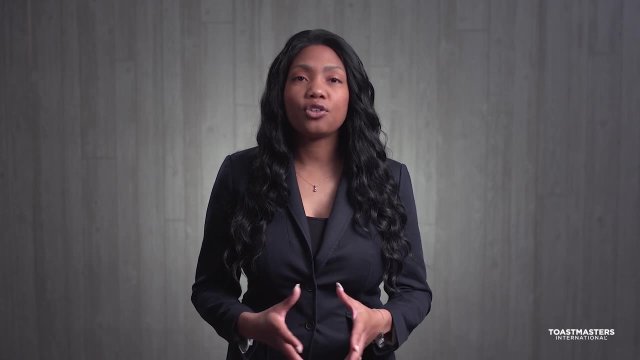 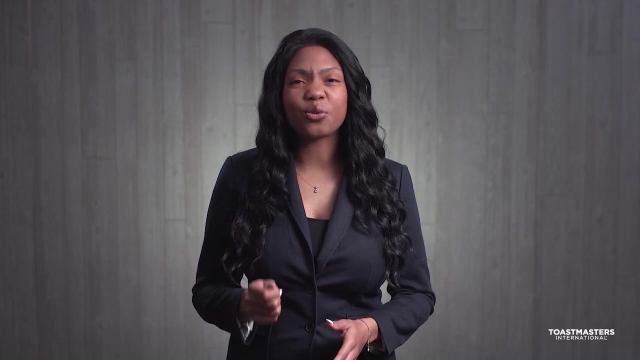 make. An advanced speaker knows how to guide the audience's attention toward the important parts and away from the small stuff. Whether you make a mistake or not, just remember that people want you to succeed and because of that, they're rooting for you. 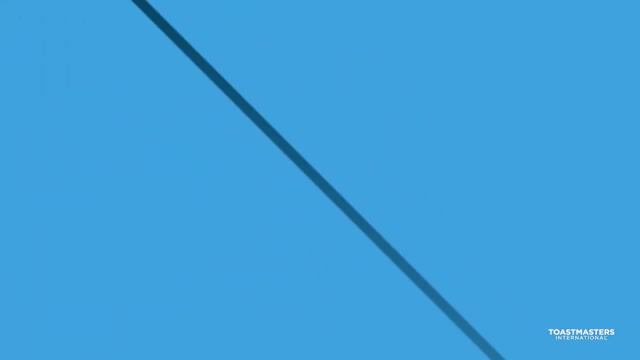 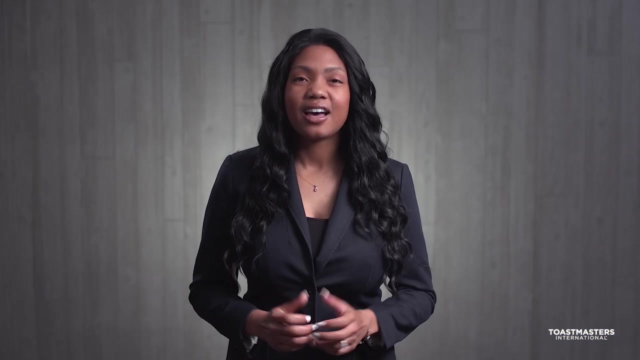 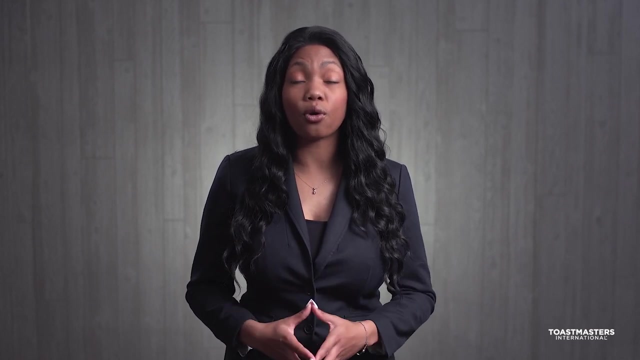 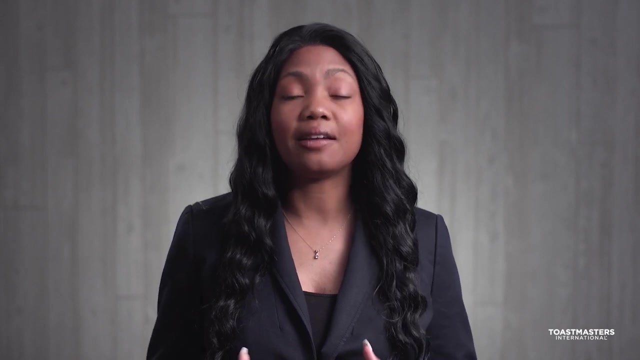 It helps to remember this with the next tip: 4. Imagine yourself giving a great speech. A great way to find success is to visualize it. Give yourself time for this important form of preparation. See yourself making clear, valid points with appropriate gestures and body language. that 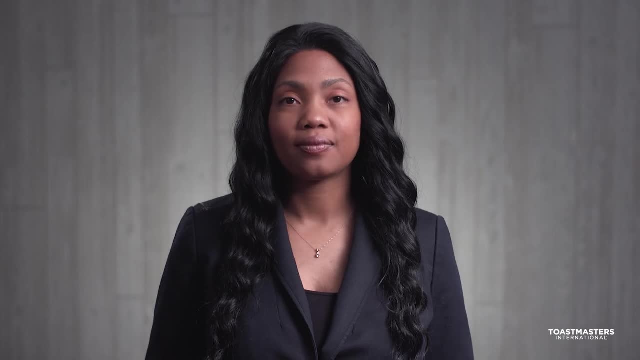 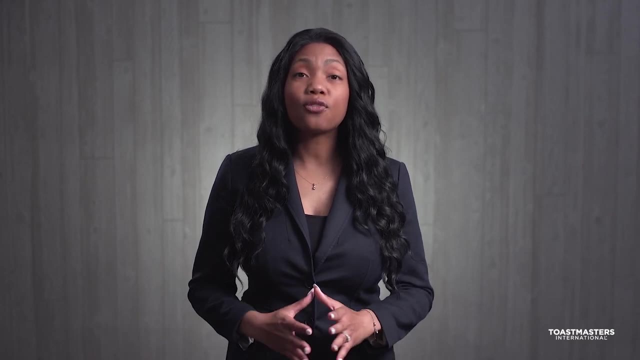 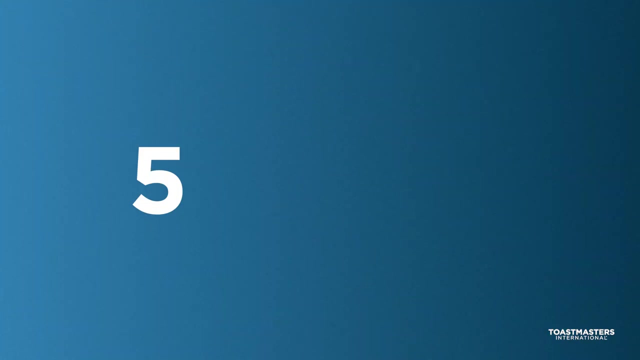 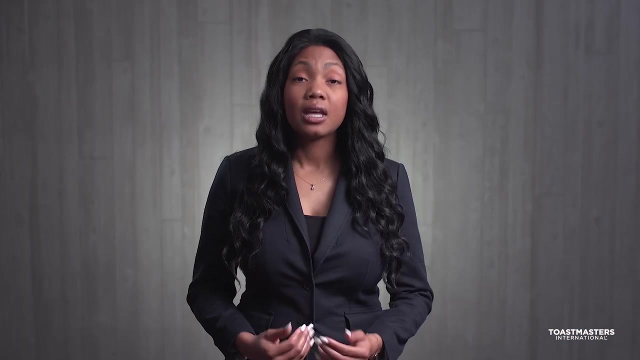 emotionally connects you with your audience. Once you see yourself using what works, you'll feel more relaxed and confident. And don't forget to imagine pausing while your audience applauds wildly. 5. Focus on your message, not on yourself. Some beginning speakers let their nervousness win because they make the mistake of focusing.